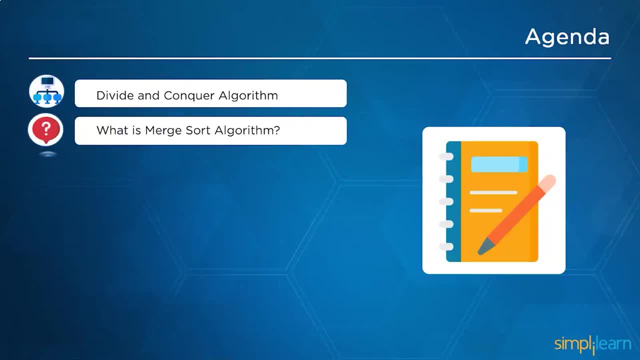 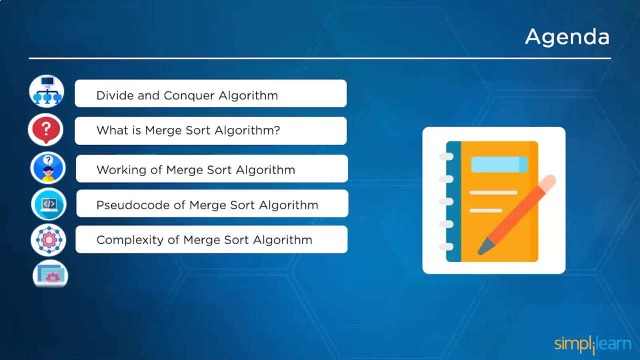 we will try to define the Merge Sort algorithm. After that we will understand the working of Merge Sort algorithm. Later we will learn the pseudocode of Merge Sort algorithm. After that we will understand the complexities of Merge Sort algorithm. Next we will see. 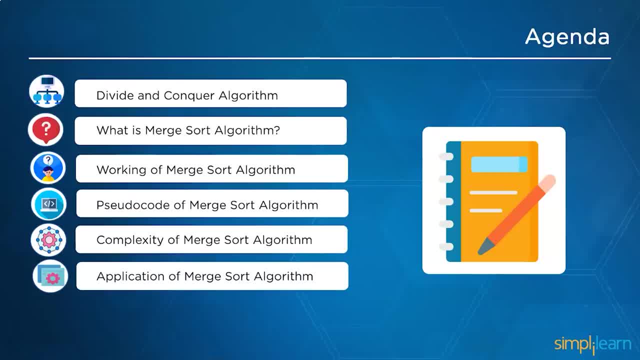 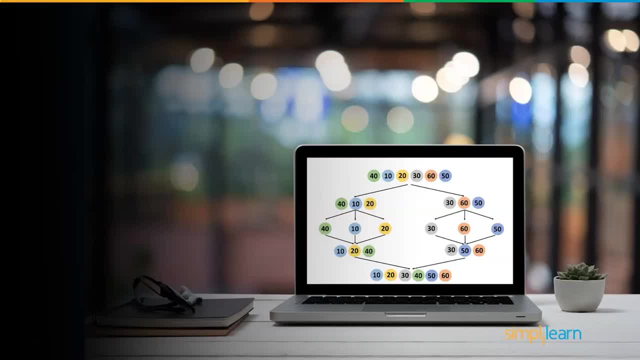 some of the real-time applications of Merge Sort algorithm. And finally, we will wind up the session by understanding some of the important drawbacks of Merge Sort algorithm. But before we begin, let me tell you a little bit about Divide and Conquer algorithm. 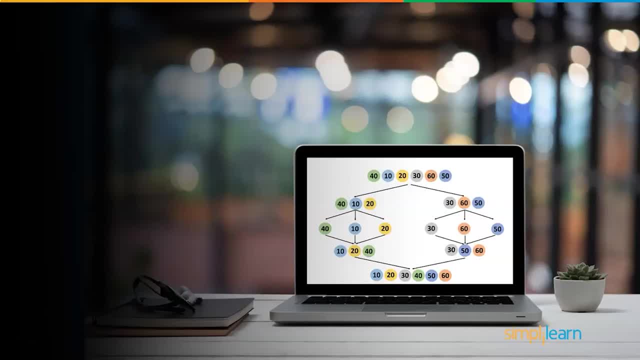 Let me tell you, guys, that we have daily updates on multiple technologies. So if you are a tech geek in a continuous hunt for latest technological trends, then consider getting subscribed to our YouTube channel, and don't forget to hit that bell icon to never miss. 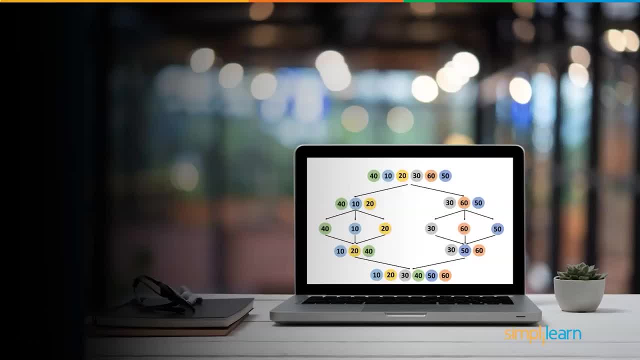 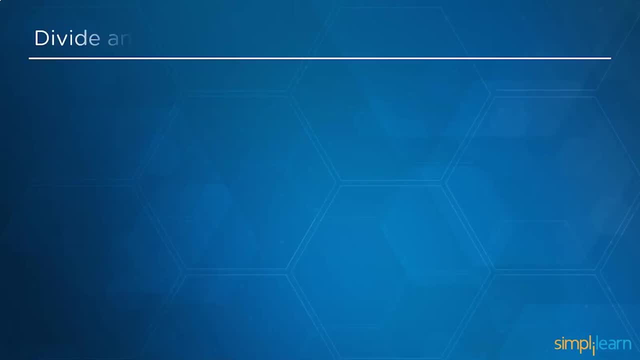 an update from Simply Learn. So, without further ado, let us get started with our first topic, that is, what exactly is Divide and Conquer algorithm? A Divide and Conquer algorithm iteratively divides a problem into two or more sub-problems of the same or relative. 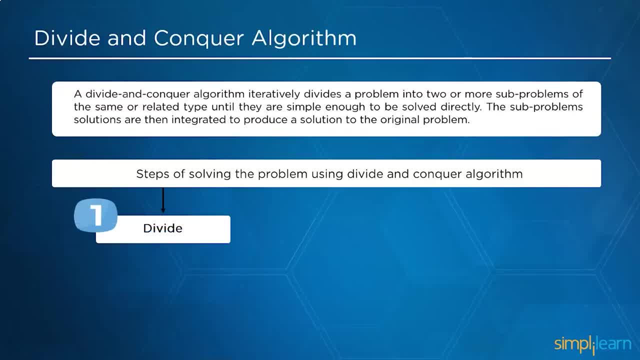 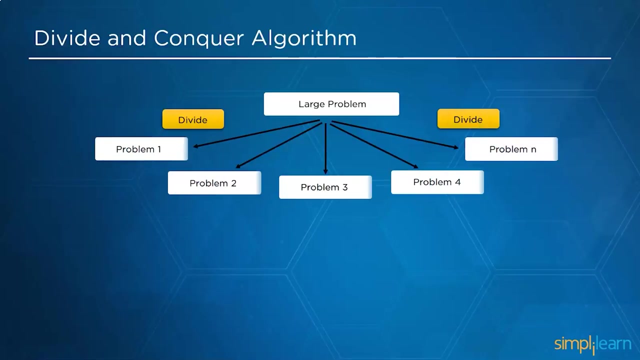 type, For example. they are simple enough to be solved directly. The sub-problem solutions are then integrated to solve the original problem. There are three steps involved in the Divide and Conquer principle, that is, divide, conquer and combine. The first step is to divide the significant problem into smaller sub-problems. 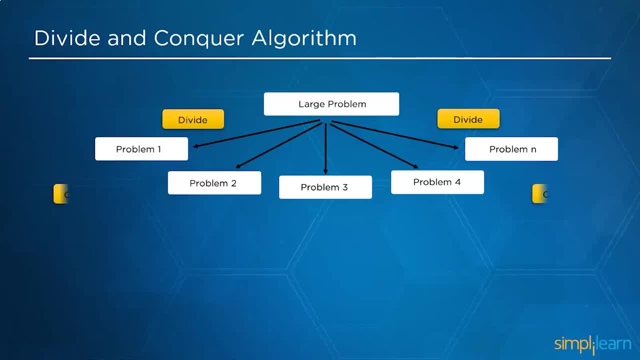 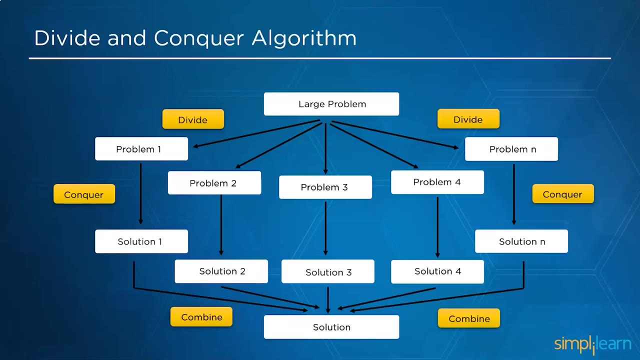 The second phase is to conquer the solutions to all divided sub-problems. Then the final step is to combine and merge all of the solutions to create a definite solution. We will understand this by an example right here on my screen. Suppose we have a large problem. we can use divide and conquer technique to divide. 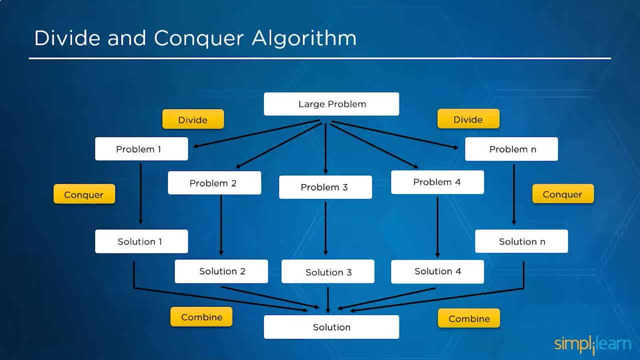 it into N number of sub-problems, Such as problem 1, problem 2, problem 3, problem 4, and so on. Until we reach problem N, Then we conquer all the solutions to specified sub-problems, as solutions such as 2 to 2 to 1 to n to 1 to 2 to n to N. Solution1PLじゃ. 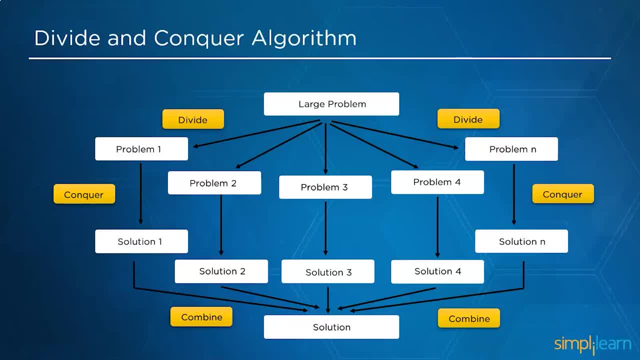 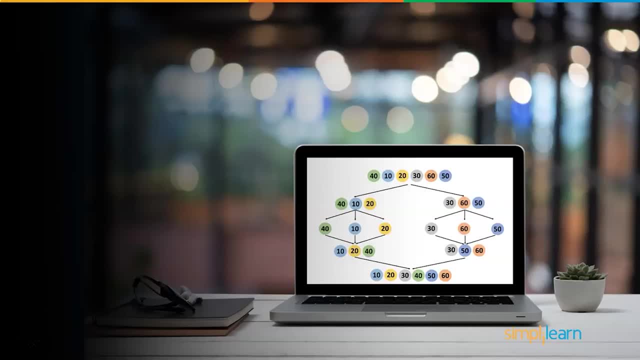 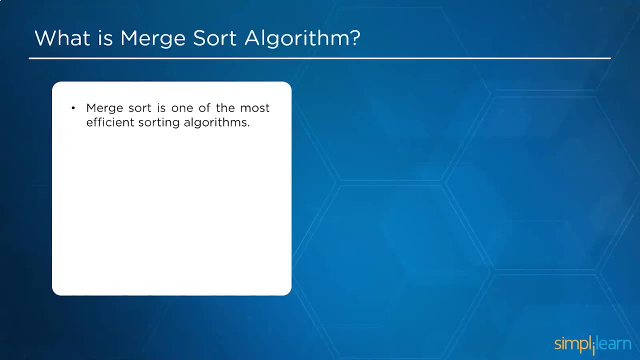 3, 4 and so on, and finally we merge all the solutions to get one definitive solution. Now, that was divide and conquer algorithm. followed by that, Let us get into much sort algorithm. So much sort is one of the most efficient sorting algorithms. It is based on divide and conquer strategy. 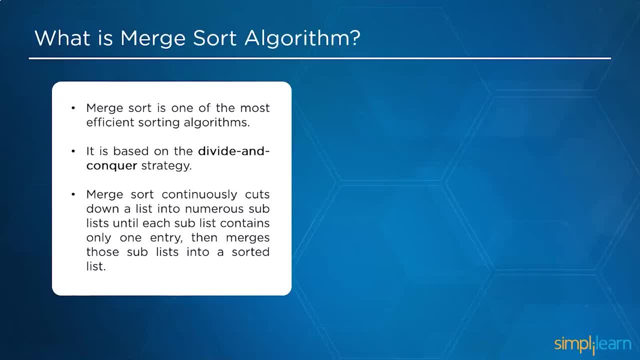 much sort, continuously divides a list into numerous sub list until each sub list contains only one entry, then Merges all those sub lists into a sorted list. There are four elements on my screen. We have seven and three in the left half and five and two in the right half. 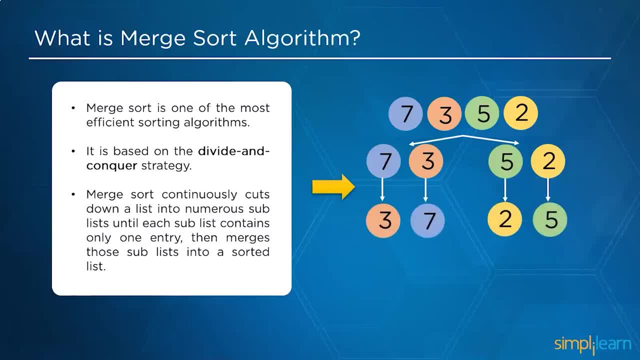 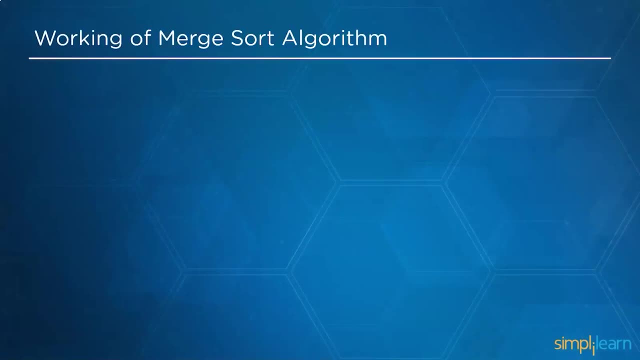 After dividing the four elements in half, we combined all the items in ascending order, that is, two, three, five and seven. In the next segment we are going to understand how It happened and we are going to learn the working procedure of much sort algorithm. There are two approaches to implement the Merge sort algorithm. 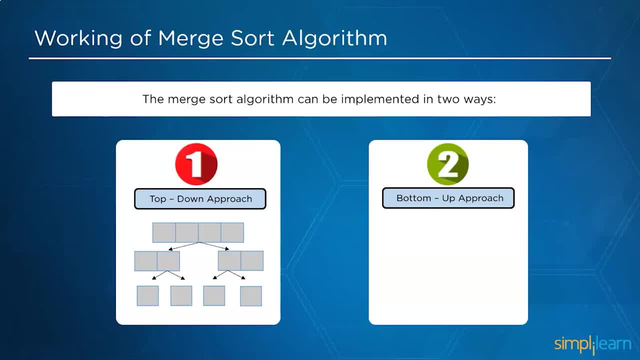 The first method is top-down approach and the second method is bottoms-up approach. The first method, that is, the top-down approach, implies that it begins with the large picture. from then It's broken into smaller chunks. Now the second method, that is the bottom-up technique, which starts with a specific number of jobs and works its way up. 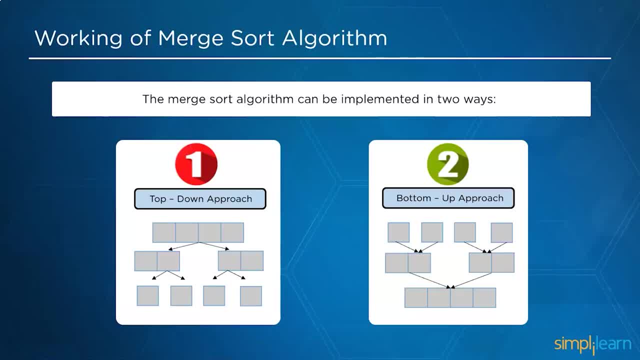 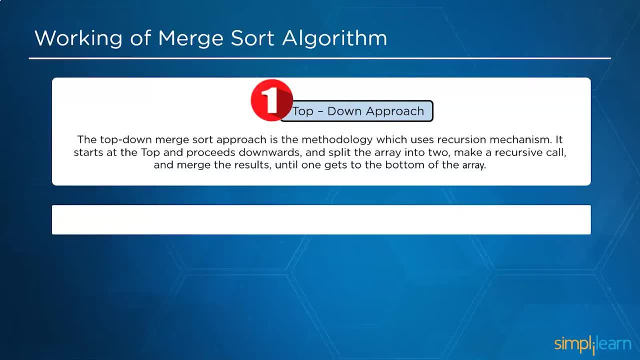 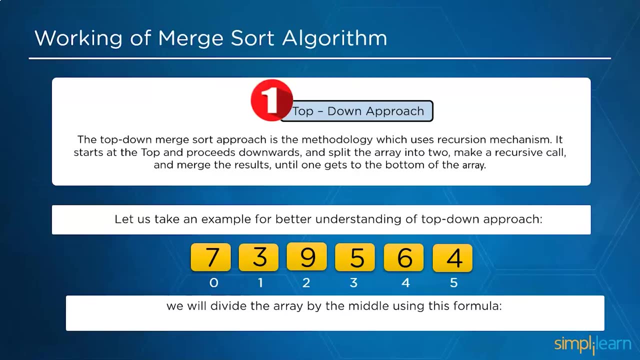 to the general. Let's have a look at how to implement the Merge sort algorithm using top-down approach. The top-down Merge sort approach is the methodology that uses a recursion mechanism. It starts at the top and proceeds downwards, splitting the array into two halves, Making a recursive call and merging the results until one gets to the bottom of the array. for a better understanding of the top-down approach, 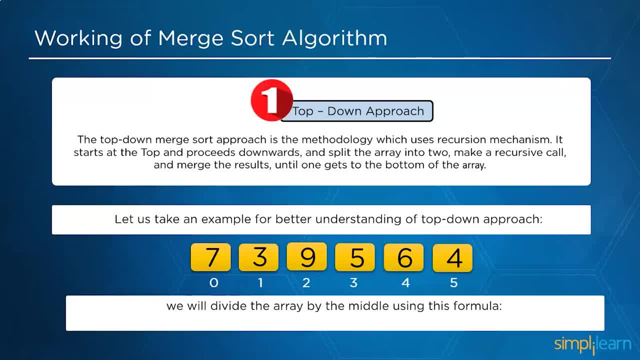 method. Consider the following scenario. right here on my screen We have an example of an array of size 6 consisting of elements 7, 3, 9, 5, 6 and 4, Starting with 0 and ending with 5. Using the following formula will divide the array by its middle. That is, middle is equals to left plus right divided by 2. 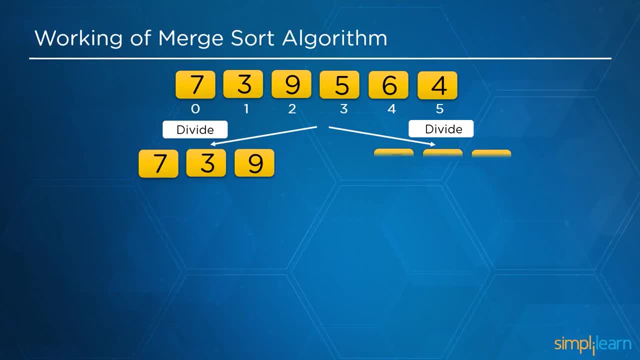 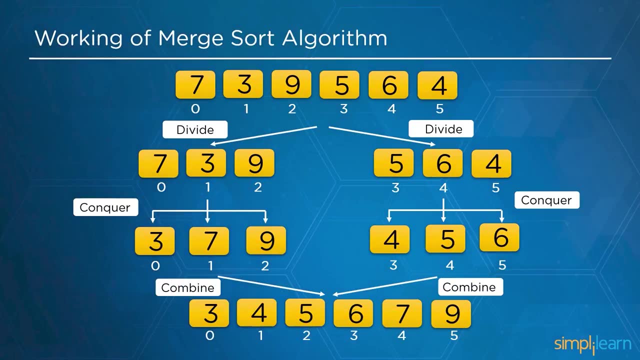 We have three elements on the left and three elements on the right, near the middle. So, according to the top-down strategy, we divide the given array in half, resulting in three elements, That is, 7, 3 and 9 on the left and 5, 6 and 4 on the right. 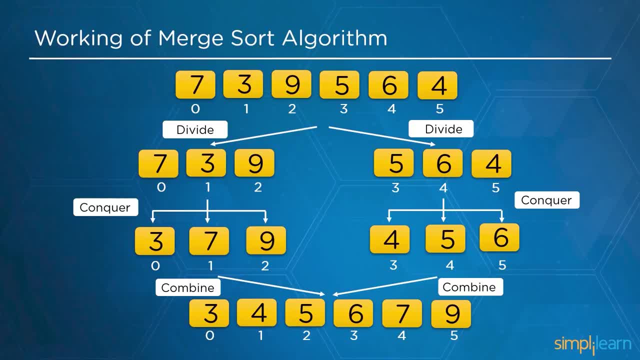 Next, we sort all these elements in ascending order. By doing so, the first half will be 3, 7 and 9, and the right half will be 4, 5 and 6, and after Merging all of them, We will have the sorted array, That is, 3, 4, 5, 6 and 9. 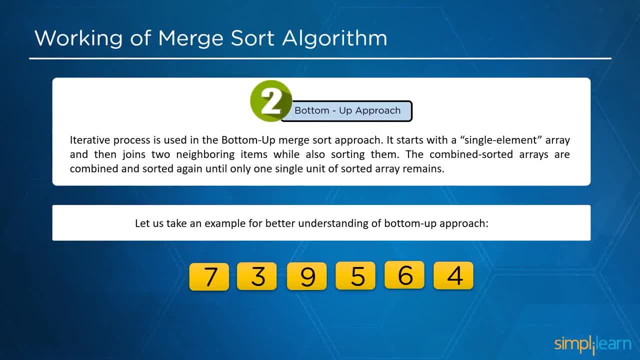 Next we will understand the bottoms-up approach. an, An iterative process, is used in bottoms-up merge sort approach. It starts with a single element array and then joins two neighboring items while also sorting them. The combined sorted arrays are combined and sorted again only until one single unit of the sorted array elements remains. 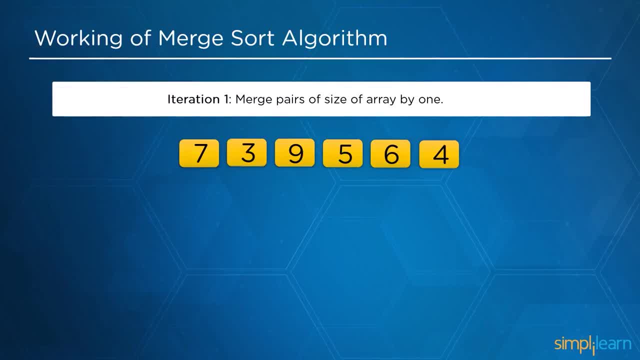 Now let us look at an example right here on my screen. in the first iteration We will merge pairs of array sizes by one, sorting each of the two elements. when you iterate the Array by size 1, the elements 7 and 3 become 3 and 7. similarly, 9 and 5 become 5 and 9, and. 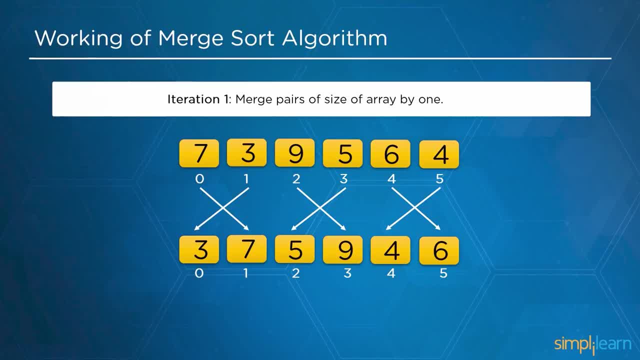 Finally, 6 and 4 become 4 and 6. We will merge the pairs of array size by 2 in the next iteration With the bottoms-up method. as a result, the elements 3, 7 and 5 will become 3, 5 and 7 and the same way. 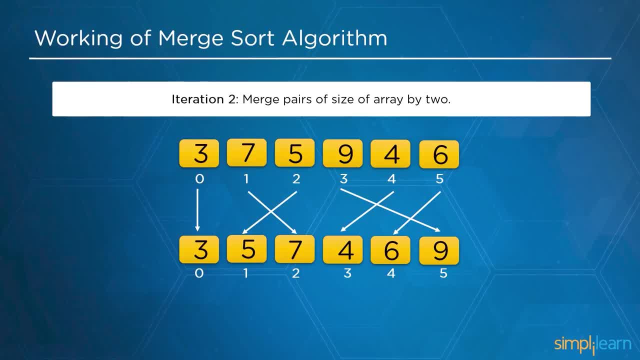 9, 4 and 6 will become 4, 6 and 9 in the last iteration merge We will merge the pairs of array size by 3 so that after sorting 3, 5, 7, 4, 6 and 9 becomes 3, 4, 5, 6 and 7 as sorted arrays. 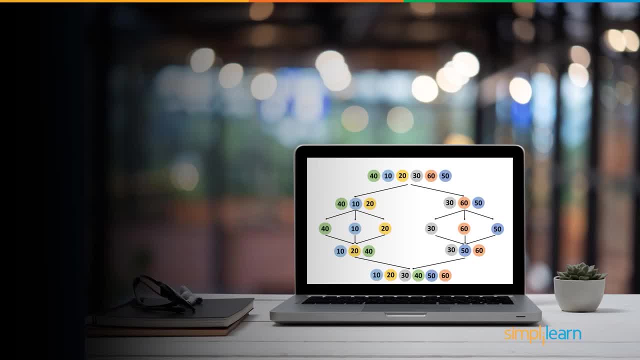 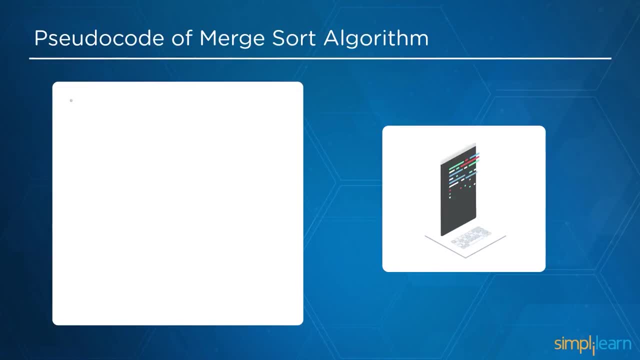 After understanding the working procedure of merge sort algorithm, We will now see the pseudo code of merge sort algorithm. We have a function called merge sort in this pseudo code, and Parameter of the function contains an array named as array and two variables named as left and right. 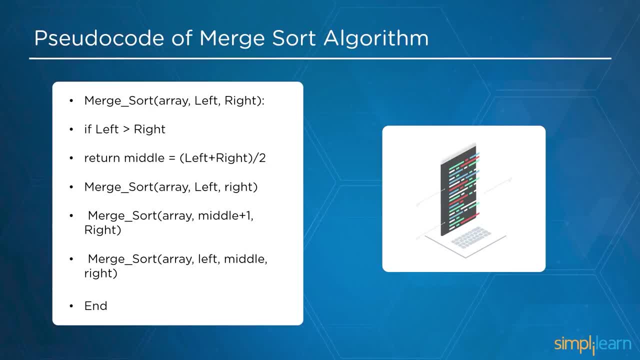 We have a function called merge sort in this pseudo code, and parameter of the function contains an array named as array and two variables named as left and right. If the number of elements in the left is greater than the number of elements on the right, We will get a middle using formula: left plus right divided by 2. 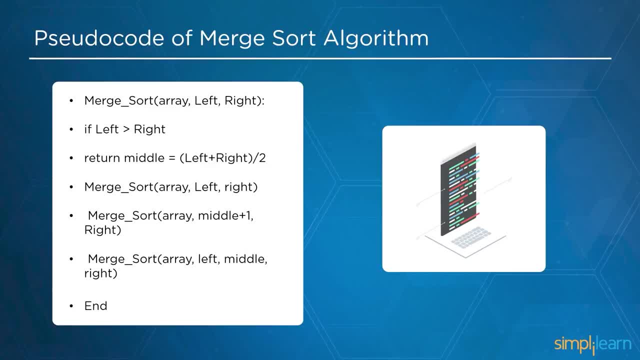 The merge sort is called and this function now has an array, a left variable and right variable. by calling merge sort, We have array left as middle plus 1 and right variable and finally, by calling merge sort, We have left, middle and right variables in our upcoming segment. 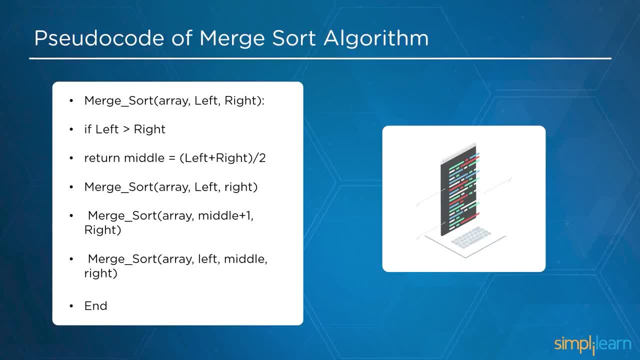 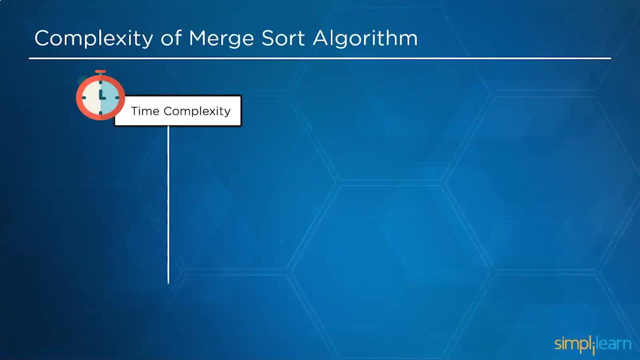 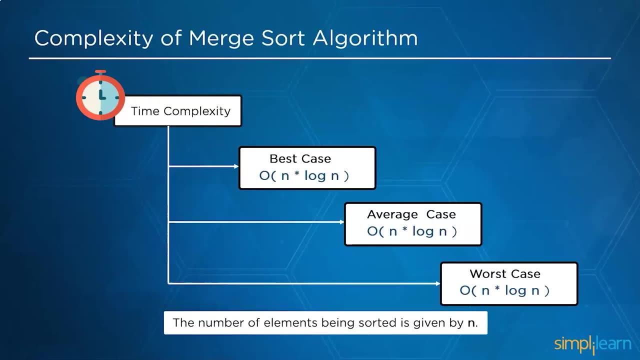 we will implement the Merge Sort method in a practical demonstration. In the next section we will discuss the complexity of Merge Sort Algorithm. First we will look into the time complexity of Merge Sort Algorithm. As we all know, time complexity in data structures is divided into Best Case, Average Case and 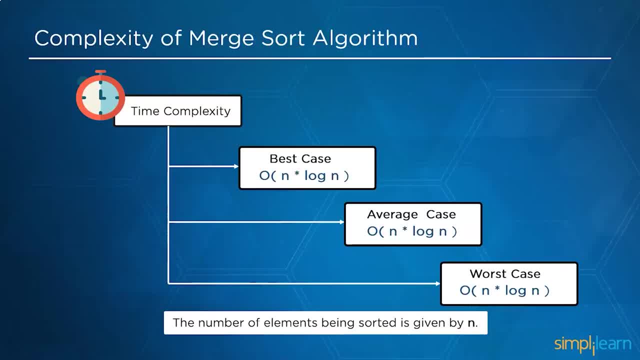 Worst Case. The best case of Merge Sort Algorithm is O into log n. Average case of Merge Sort Algorithm is O into log n And the worst case of Merge Sort Algorithm is O into log n. The number of elements being sorted is given by n. 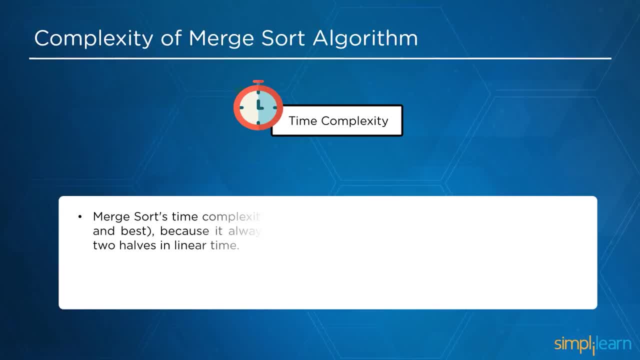 Merge Sort's time. complexity is O in all three situations, ie worst, average and best, because it always divides the array into two halves and merges the two halves in linear time, So it takes up the same amount of space as the Unsorted array. 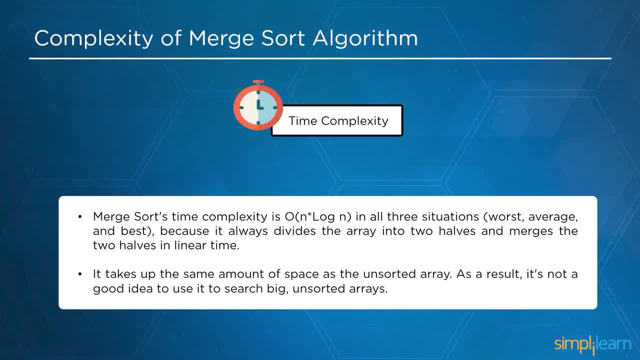 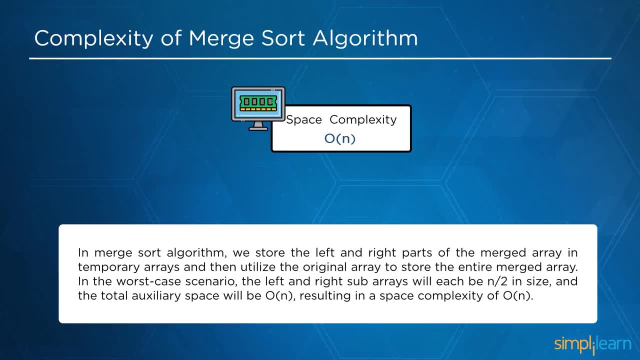 As a result, it's not a good idea to use to search big Unsorted Arrays. Moving on to the space complexity of Merge Sort Algorithm, The space complexity is large, O of n. In the merge-sort algorithm we store the left and right parts of the merged arrays. 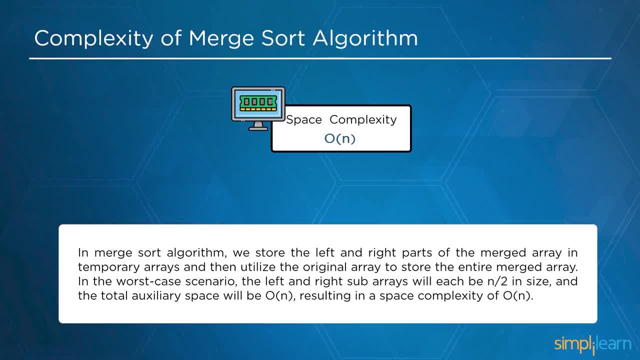 and then utilise the original array to keep the entire merged array. In the worst case scenario, the left and the right subarrays will each be n by 2 in size, and then the total auxiliary space will be O, resulting in a space complexity of O. 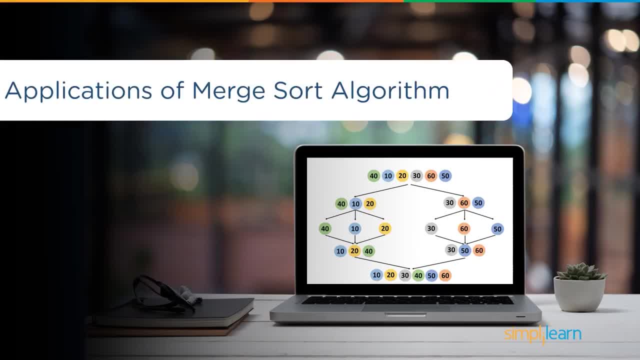 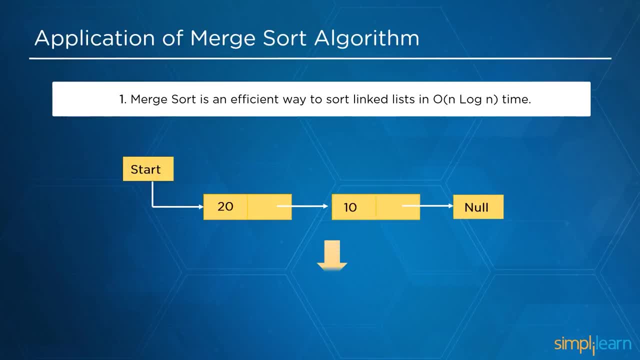 Following that, we will look into several applications of the Merge Sort algorithm. So the first application is Merge Sort is an efficient way to sort linked lists in O n log n time. Subsequent application of the Merge Sort algorithm is, for linked lists, Merge Sort implemented. 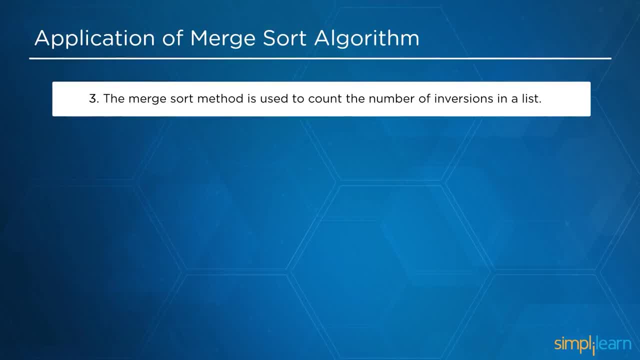 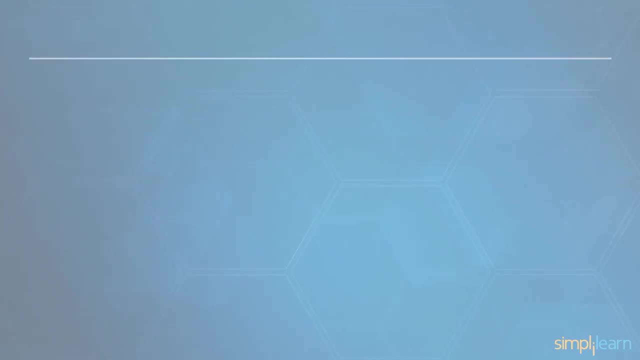 without taking up more space. Followed by that, the Merge Sort method is used to count the number of inversions in a list. Last application states that in internal sorting the Merge Sort is employed. Now let us look into some of the drawbacks of Merge Sort algorithm. 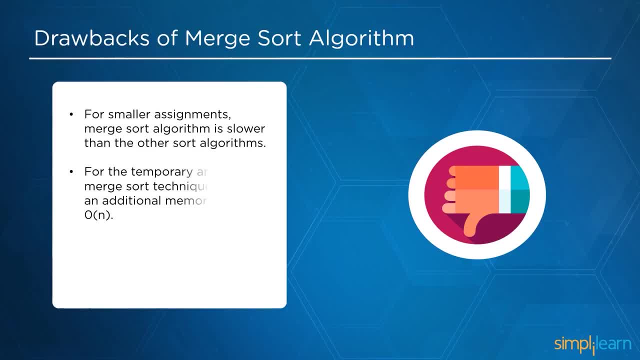 So some of the drawbacks of Merge Sort algorithm are: For smaller assignments, Merge Sort algorithm is slower than the other sorting algorithms. For temporary array, the Merge Sort technique requires an additional memory space, ie space of O. Now let us look into a practical demonstration of Merge Sort algorithm. 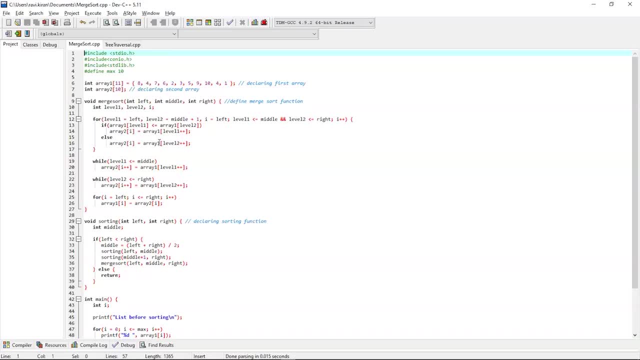 On my screen we have an example for Merge Sort algorithm To define constants or microsubstitution. we use the hash defined as preprocessor directive with a constant variable, max of 10.. Following that, two arrays, Array1 and Array2, are declared. 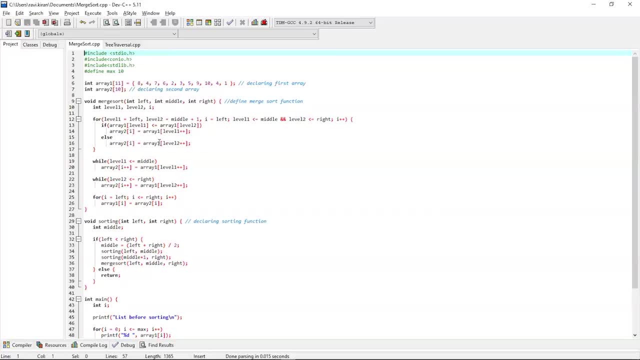 We declare Array1 and initialize it with elements like 8,, 4,, 7,, 6,, 2,, 3,, 5,, 9,, 10,, 4 and 1.. Array2 is used for temporary array. 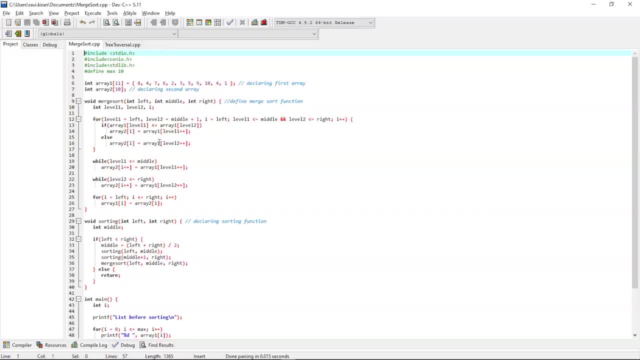 Then, to implement the Merge Sort concept, we declare a Merge Sort function. We specify three variables in this function parameter, ie left, right and middle. The left variable is used to display the array. The right variable is used to display the array. 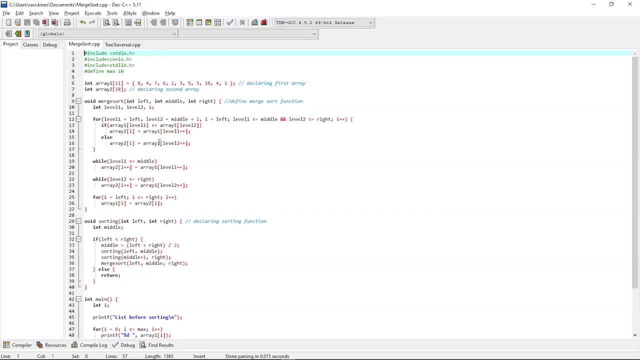 The left variable is used to display the array. The left variable is used to display the left part of the array1.. The right variable is used to display the right part of the array1 and the middle variable is used to indicate the middle or centre of the array in this function. 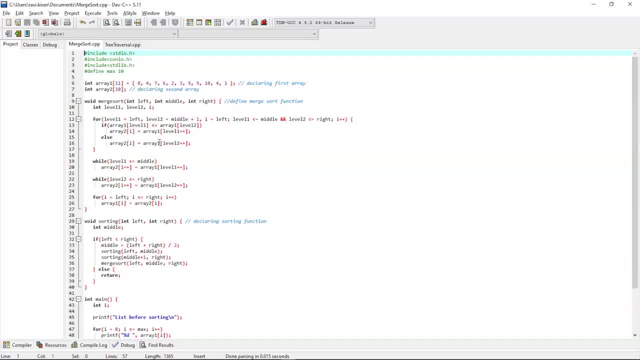 We utilize the for loop in the function setting the left to level 1, the middle plus 1 to level 2 and the left to variable i, with the condition that level2 is less than or equal to the middle and level2 should be less than or equal to the right of the array. 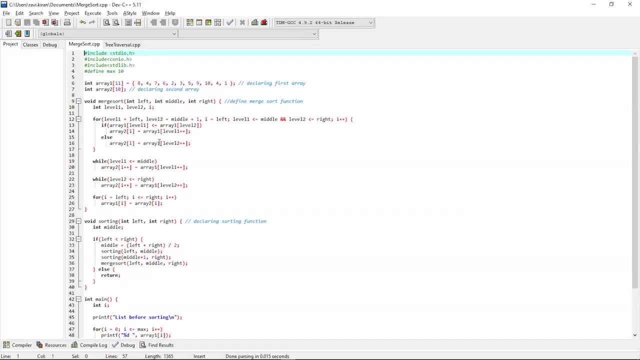 We have a condition in this for loop that if level1 of array1 is less than or equal to level2 of array1, we will initialize all the consecutive elements of level1 of array1 to array2.. Else, we will initialize all the successive elements of level2 of array1 to array2.. 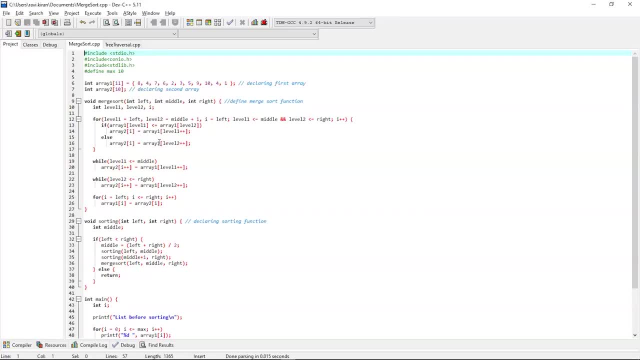 Out of for loop. all subsequent elements of level1 of array1 will be initialized to array2 until level1 is less than or equal to the middle. All successive elements of level2 of array1 will be initialized to array2 until level2 is less than or equal to the right of the array. 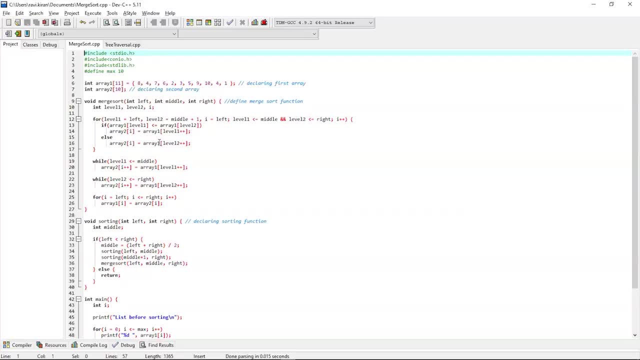 Using the loop which will run from i, equal to the left of. i is less than or equal to right. we initialize all the items of array2 to array1.. We have declared one more function in this code, namely sorting Out of the merging sort function, in which only the left and right variables are defined. 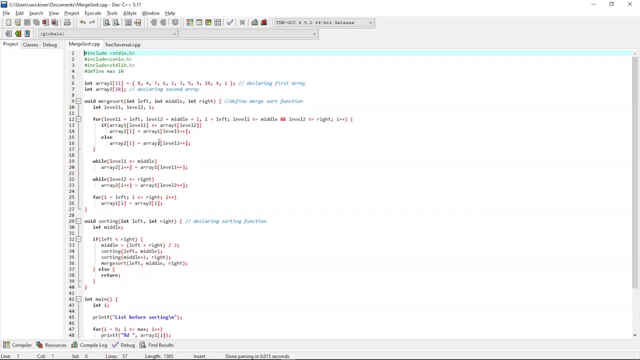 we specified the middle function in the sorting function with the condition that if the left is less than the right, the middle will be calculated as left plus right divided by 2.. Then we called the sorting function, passing left as middle, as right, and then another sorting. 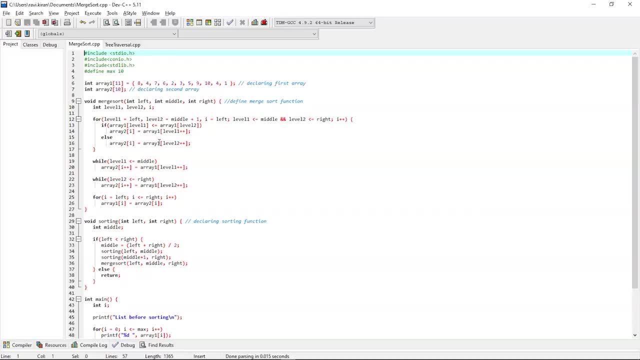 function passing left as middle plus 1 and right. Finally, we used the merge sort function, passing left, middle and right to the sorting array 1, otherwise we would return nothing. We entered the main function of sorting and we have completed the sorting function. 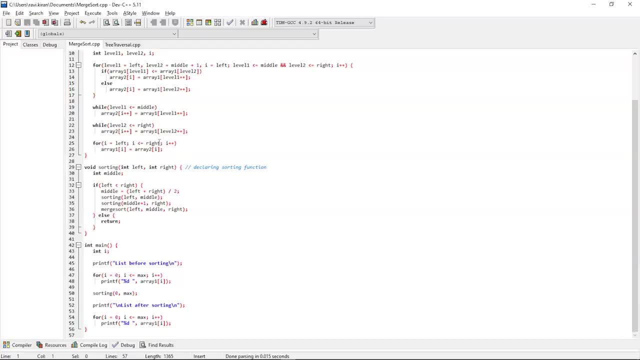 function out of the sorting function, where we declared the counter variable i and printed the array before sorting using the printf function in for loop, where i will run from index 0 to the array's maximum size. After that we invoke sorting method, passing left as 0 index number and right as the array's. 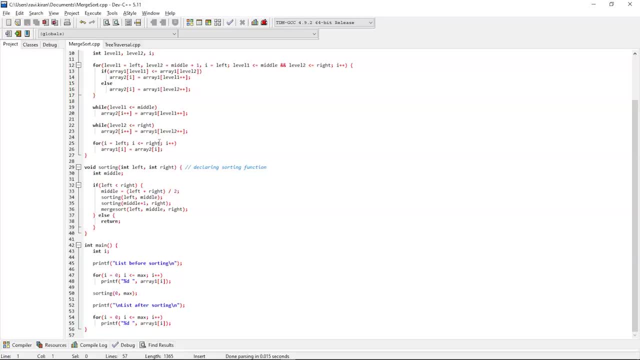 maximum value. Finally, after doing the merge sort process, we will print the array using the printf function and for loop We will run from 0 to the array's maximum value. Then we compile the program and run it. Now let's try to quickly execute this program and see the output. 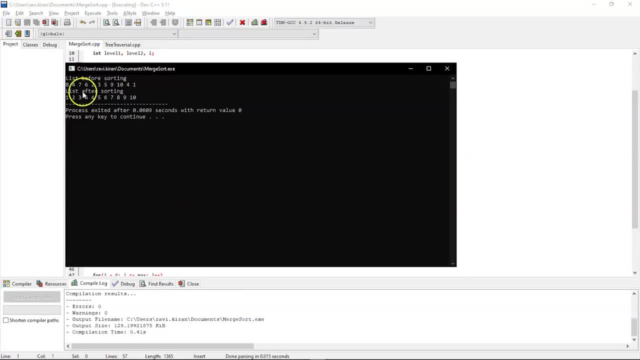 So there you go. the program got successfully executed and the list before sorting is 8,, 7,, 6,, 2,, 3,, 5,, 9,, 10,, 4 and 1.. And the list after sorting is 1,, 2,, 3,, 4,, 4,, 5,, 6,, 7,, 8,, 9 and 10.. 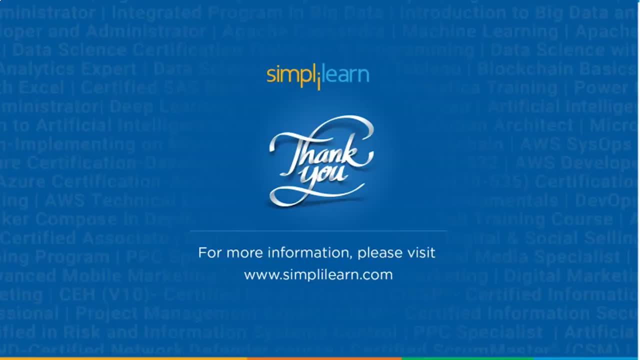 And with that we have come to an end of this session on merge sort algorithm. If you have any queries or if you need the code executed in this particular tutorial, then please feel free to let us know in the comment sections below and our team of experts.